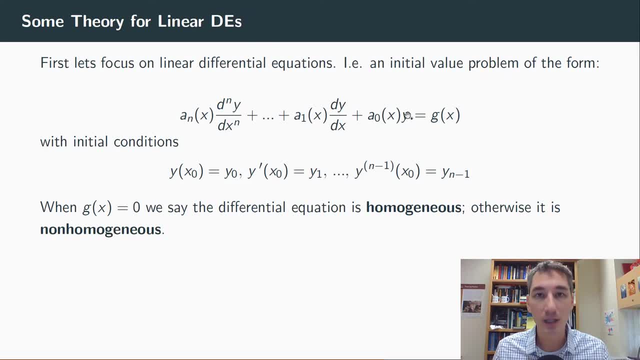 first derivative and then the function. that would be a third order. So nth order in general starts with the nth derivative down to the original function y. The fact that it's linear means that each one of those derivatives is by itself. Okay, so you're never multiplying the. 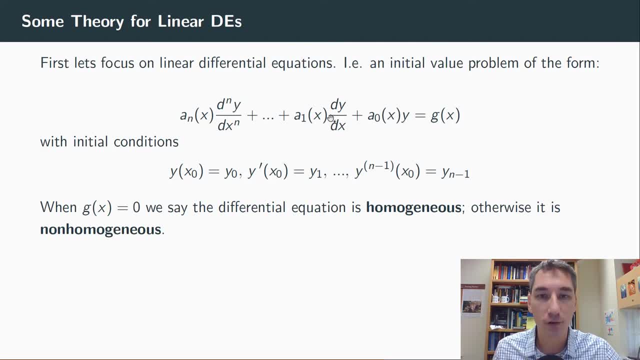 first derivative times the function or anything like that. It's just the function, the first derivative, on up to the nth derivative. If it is multiplied by something, it's only a function of x or t, whatever the independent variable is. So here we have some function of x times the nth. 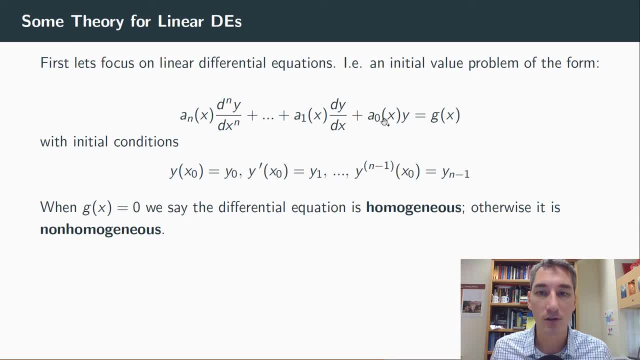 derivative, some function of x times the first derivative, some function of x times the function, and then set equal the right hand side, which is just a function of x. Okay, so that is, when we say a, you know a second order linear differential equation, it should be a2 of x. 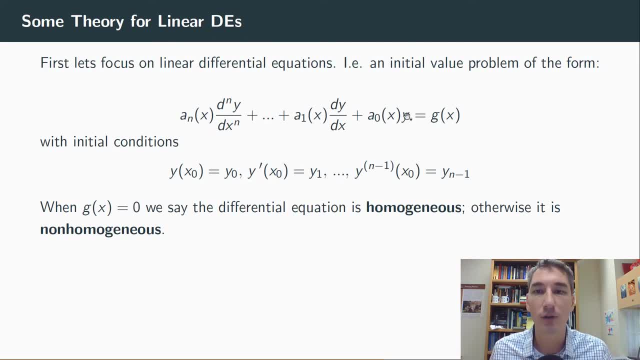 2y, a1 of x, dy, a0 of x, y, g of x. Okay, it's an initial value problem because we specify the initial condition, so initial position, initial velocity, initial acceleration on up to the nth derivative right or the n minus 1 derivative. So because we start at y, 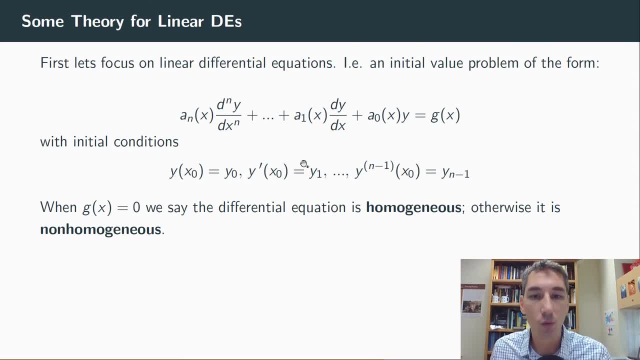 initial position, which is 0,, and then 0,, 1,, 2, up to n minus 1,. there are n conditions for an nth order Differential equation. so a second order would have two conditions, you know: y and y prime. 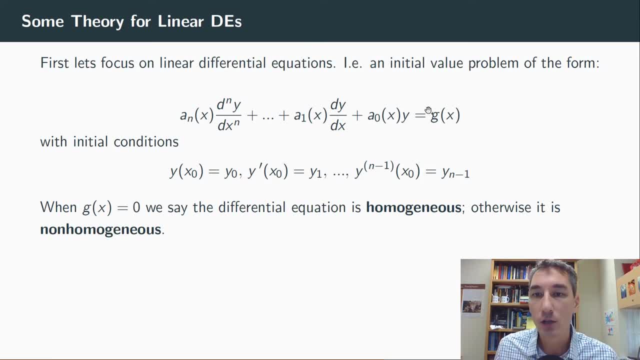 etc. Okay, now let's look at right hand side. You could have a function there, the g of x, or it could be 0. If it's 0, we call it homogeneous, otherwise we call it non-homogeneous. 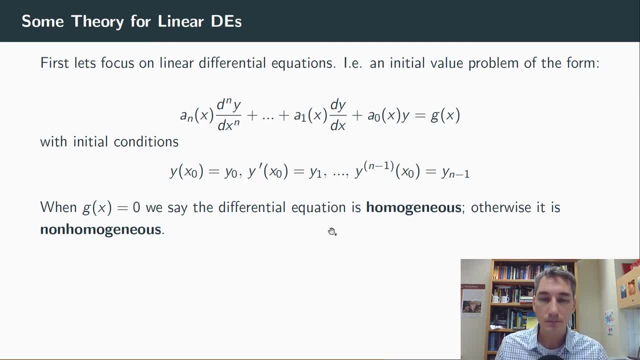 Okay, so that's what those words mean. So we could have homogeneous or non-homogeneous nth order linear differential equation, and we're going to be able to solve these if they're not too complicated. When g of x is 0, it's easier. When g of x isn't 0, it's harder, but we'll be able to handle both. 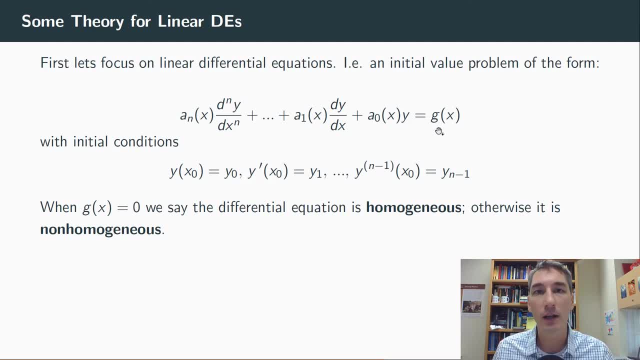 cases most of the time, And one of the things I want to just mention here: in the modeling cases this is often called the forcing term. In general, this equation here is the modeling portion, So some situation is modeled here and then this is external forces. So that's kind of how the